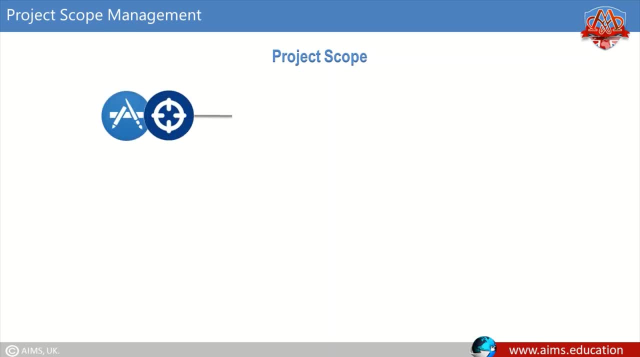 Project Scope. The Project Scope is the work performed to deliver a product, service or result with the specified features and functions. The Project Scope is all about the project and it is also known as Scope Statement. It defines the requirements of products, the work required to create the product, and it defines what is in the scope and what is not. 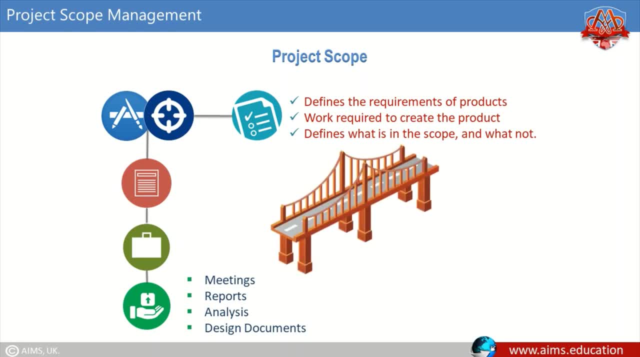 For example, if you have been given a project to build a bridge, in this case, the Project Scope will tell you what exactly you need to do to build the bridge, not anything else. See an example to understand the difference between Product Scope and Project Scope. 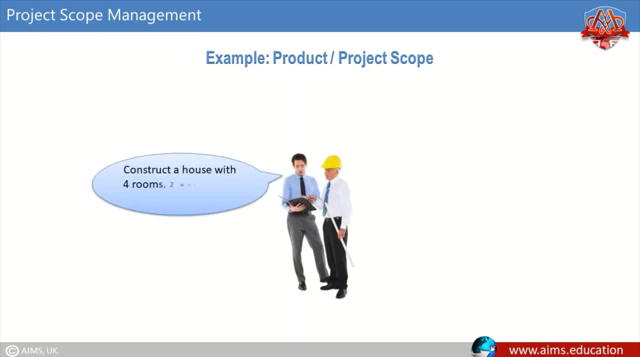 A client comes and asks you to construct a house with four rooms, two washrooms, a kitchen and a balcony. This is the Product Scope. Now you take the project and start working on it. You make the plan, create the schedule. 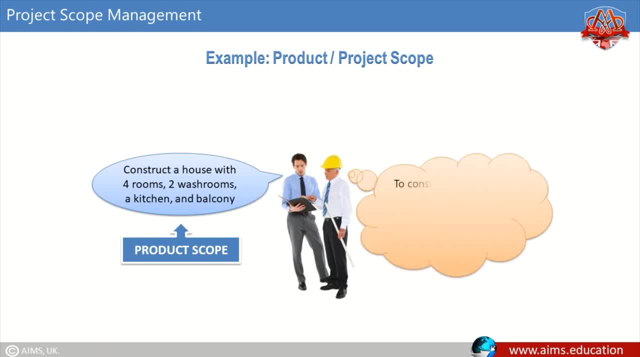 and estimate the budget. Now you finally conclude that to construct a house with four rooms, two washrooms, a kitchen and a balcony within six months, in an estimated budget of $65,000, using labor machinery and other resources, 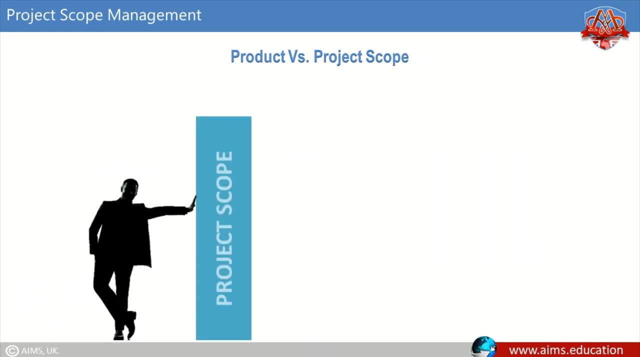 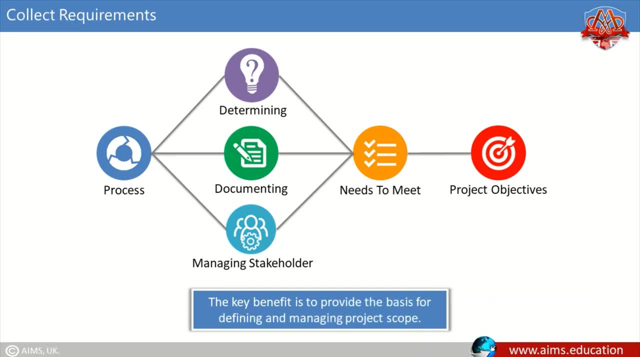 It is the first process in the project's scope. It is the first process in the project's scope and managing the project scope. including the project scope, its requirements, includes the quantified and documented needs and expectations of the sponsor, customer and other stakeholders. all of these requirements must be analyzed and recorded in a clear and detailed way to be.